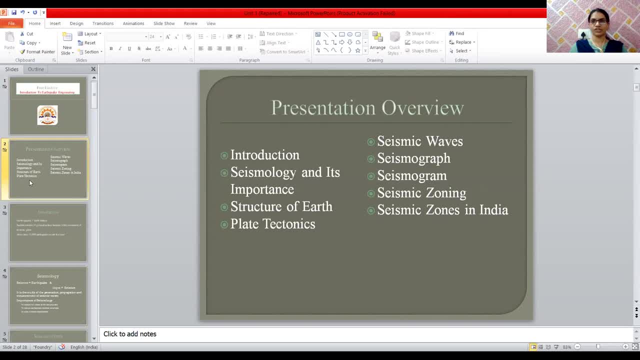 Next topic was teach in plate tectonic theory. Next seismic waves. Next topic was seismograph, seismogram, seismic zoning of India. Last topic was discussed above. First topic was introduction of earthquake. What do you mean by earthquake? 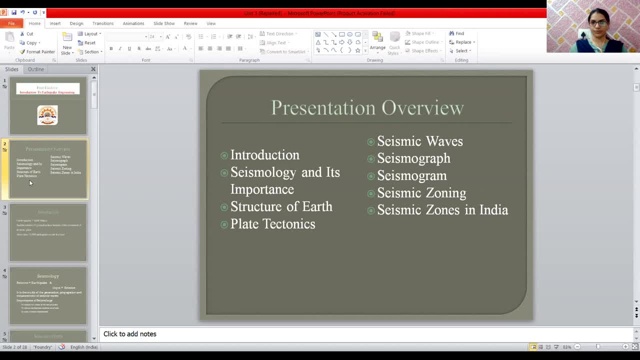 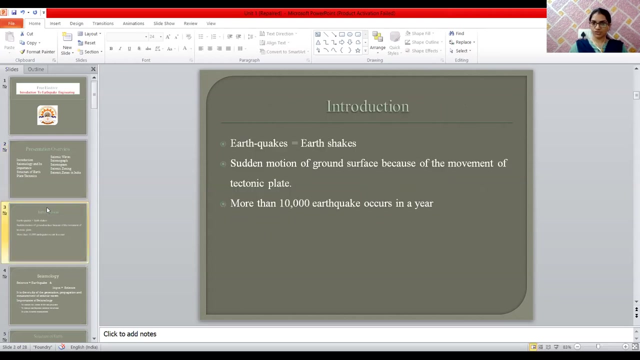 Earthquake is a sudden motion of ground surface because of movement of tectonic plates. Okay, And in simple word, the earthquake are similar words for earthquake is earth shaking. These are the similar word of earthquake, The simple language. in simple language, definition of earthquake was sudden motion of ground surface because of movement of tectonic plates. 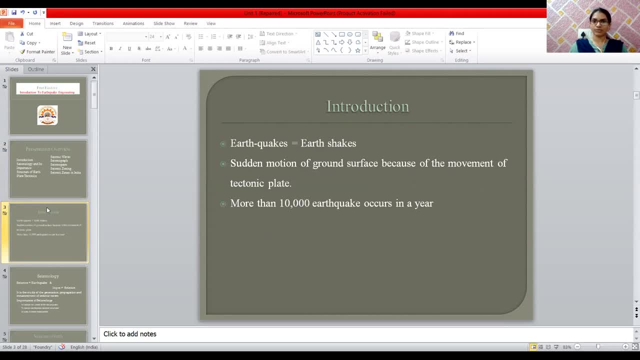 These are the simple, simple definition of earthquake. Nowadays, the in this whole earth we are more than 10,000 earthquake occurs in one year On whole of earth. more than 10,000 earthquake occurs in one year. Now we are discussing about the seismology. 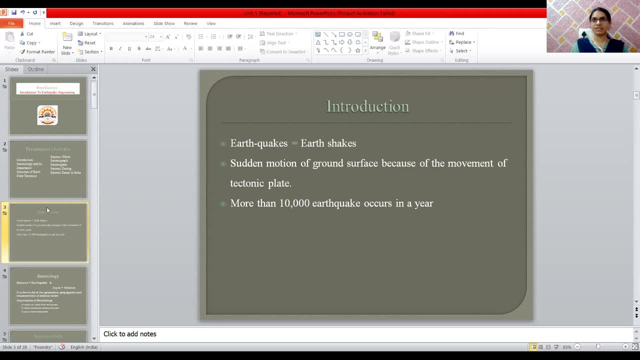 Seismology. what do you mean by seismology? Seismology means this earthquake sands. Sismo means earthquake, Sorry, earthquake, And logi in logi is a similar word for sands. In this seismology, we are studying about the graduate and propagation of propagation of waves or measuring of seismic waves. 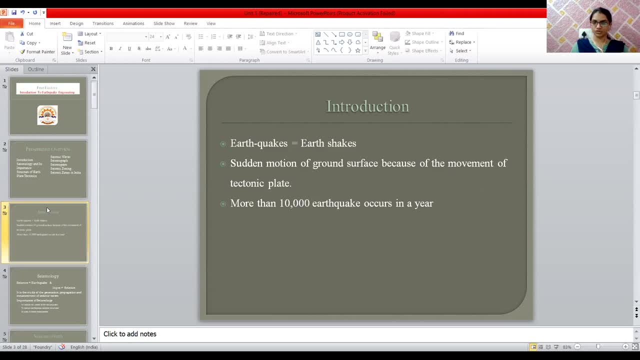 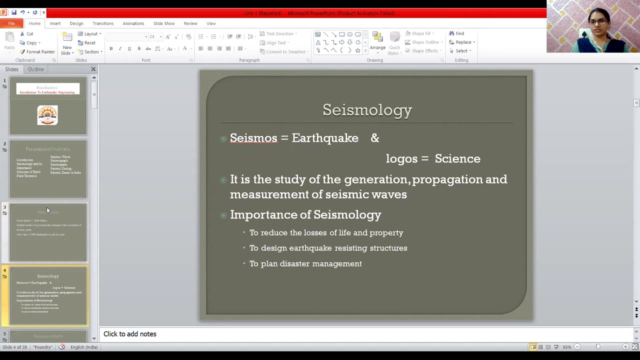 We are discussing about seismology or explain in this seismology. Seismology is very important for reduce the losses of property and less disaster, and more about these are the importance of seismology. See the seismology is similar word for earthquake. 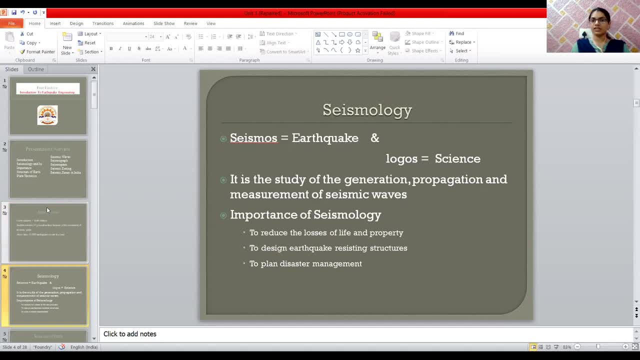 And logi is similar word for sands. It is study about the graduation and propagation and measurement of earthquake waves. These are the importance of seismology. Next topic was study the innermost part of earthquake or structure of earth In this three layers of earth. 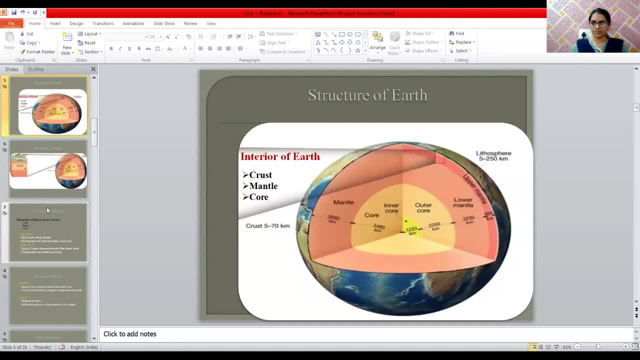 First crust in this, In this, In this diagram, we are Seen the three types of, three types of part in earthquake, In Under the ground. First crust: This is: this is topmost part of earth. Next, middle, most part of earth is mental. 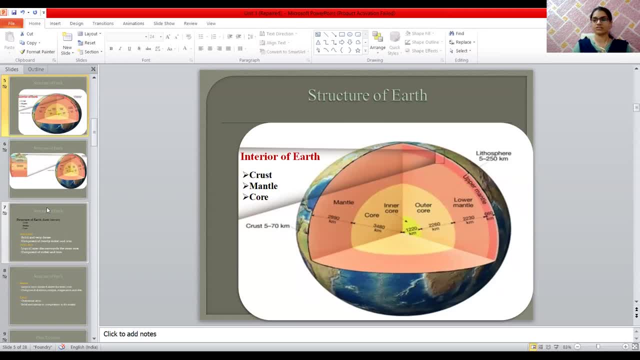 And last innermost part of earth is Core. The core has been two parts, divided into two parts. In first part we are divided into innermost core and outermost core. In this diagram we are seen about That Innermost and outermost part of earth. 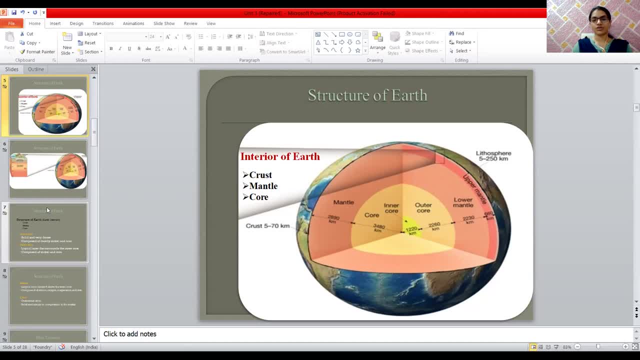 Inner core and outer core. Then mental are also divided into two parts. First, lower mental and upper mental, And core is the top, is more Topmost part of earthquake. Sorry earth, The. in this diagram we are Seen about the distance of 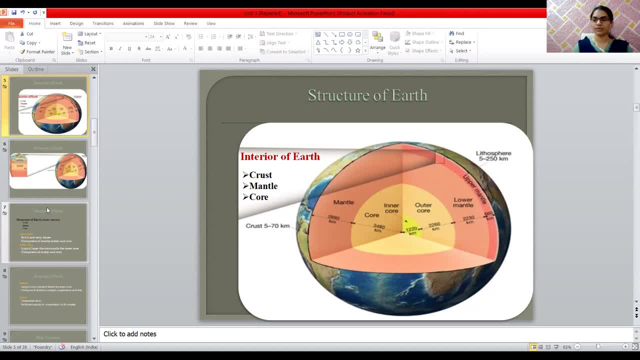 Innermost part, Outermost part, Lower mental, Upper mental and crust. These are the Distance of Earth Innermost core, Outermost core And earth Innermost core are Inner part of Earth. These are Large. 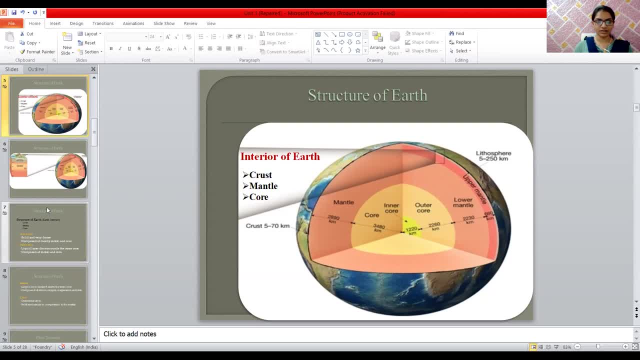 Layer, about Largest layer, about Inner core. It is composed by Silicon and Silicon and nickel Discomposed by silicon, Or sorry, Iron and nickel Discomposed by iron and nickel, And it is solid like structure. Okay, And outer core was: 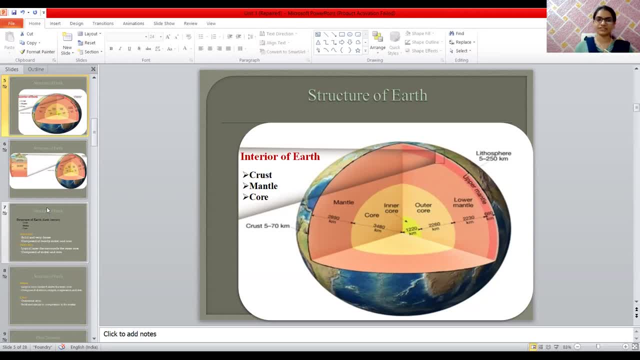 Same, Solid like structure And composed by nickel and iron. Next The mental Lower mental Lower mental At liquid like structure. Liquid like structure. Then It is composed by Silicon Oxygen And magnesium And iron. This is 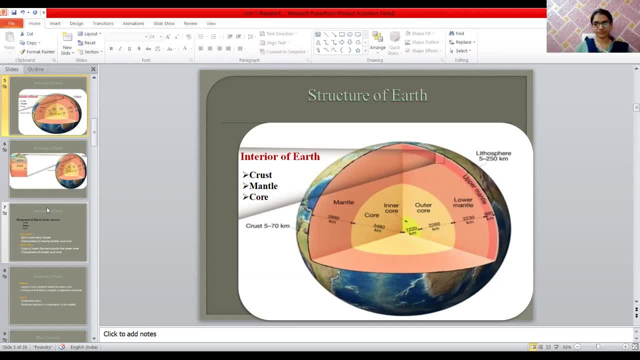 Composed by This And Upper mental Was Outer Composed by Solid, Solid like structure And it is Composed by Same Same Layer, Same Silicon, Magnetic, Oxygen And iron. This is 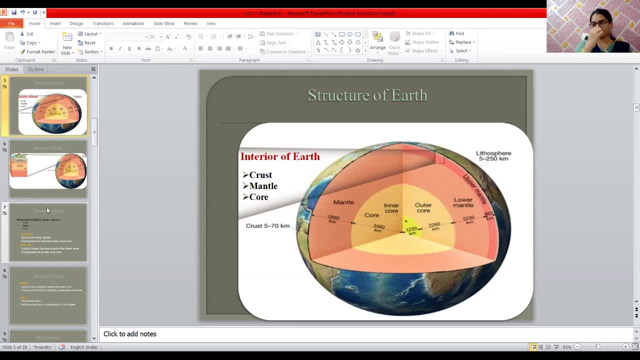 Composed by This And Upper Same: Silicon, Magnesium And oxygen Or Iron, And Outermost part of Earth, Earth Are Crust. These are, These are the Topest part of 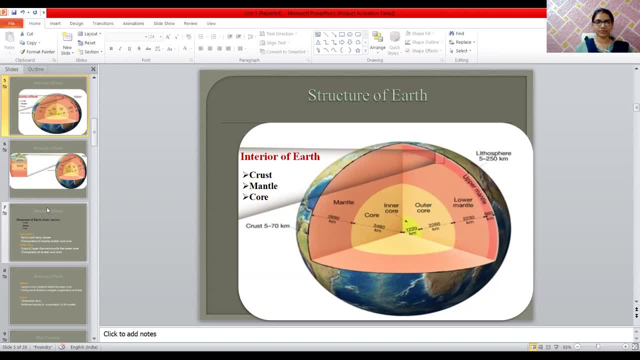 Earth And It is composed by Composed by Similar Mental Like Silicon, Iron, Oxygen And Magnetic. Okay, In this diagram We are Discussing About This First Same Diagram. 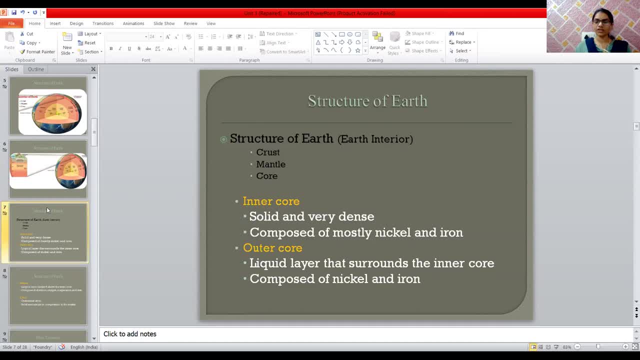 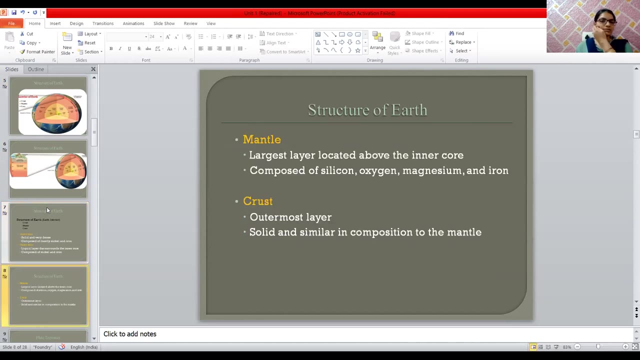 We are Discussing. See, These Are The Three Types Of Earth- Innermost Part Of Earth, First Crust, Mental- And These Are The Also Two Types. 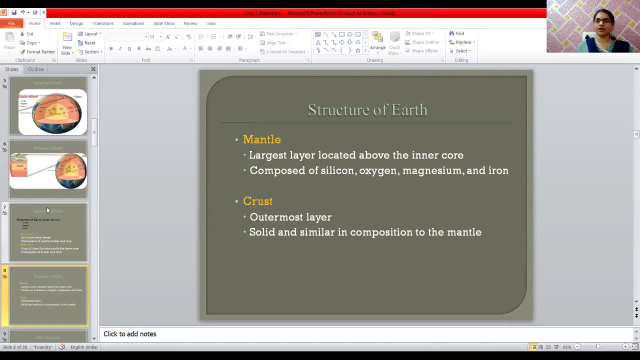 Of Mental- Outer, Outer Mental And Lower Mental And The Components Of Compo Composed By Mental Was Composed By Silicon, Oxygen And Magnesium. These 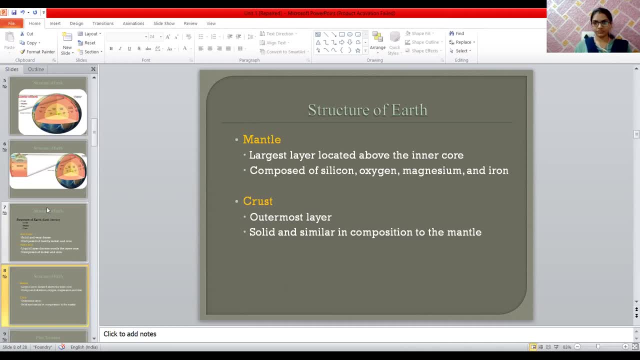 Are The Innermost Part Of Earth, And Now We Are Discussing About The Plate Tectonic City. What Even By Plate Tectonic, Plate Tectonic. 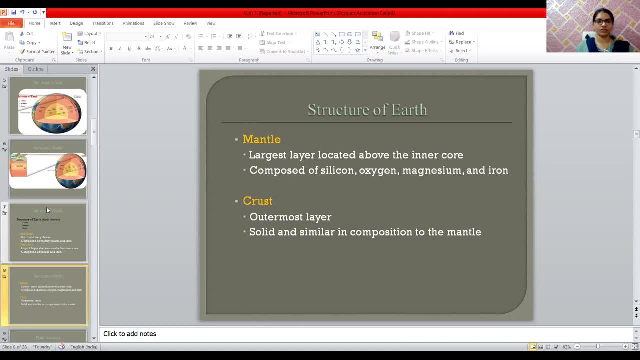 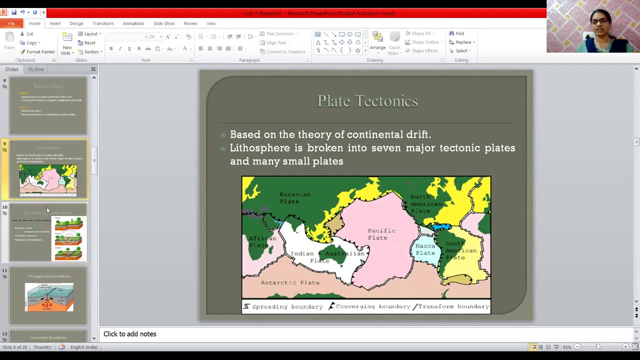 Plate Was. These Are The Plates. These Are The Plates In The. See This In This Diagram. We Are Seeing The Various Types Of Plates In. 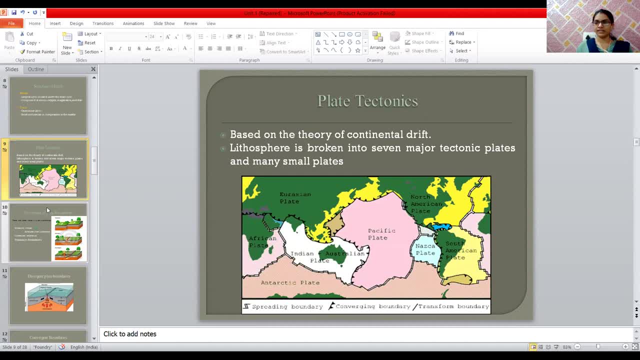 General. First Of All, Plate Tectonic Theory. Is The Plate Tectonic Theory We Are Discussing, The First Of All In Thousand Million Years. 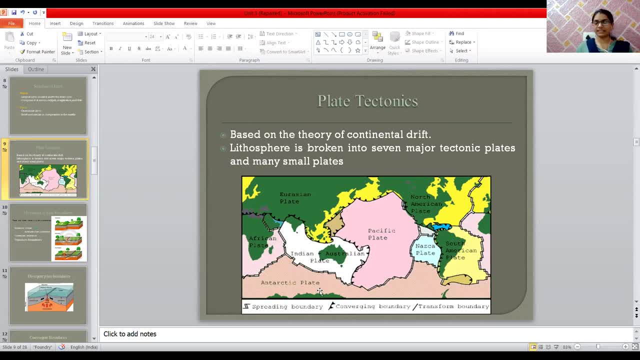 Ago The Tectonic Plate In Only Present In One Tectonic Plate. There There Were Tectonic Plates. Are Moves, Then Mapping, Are Development Or 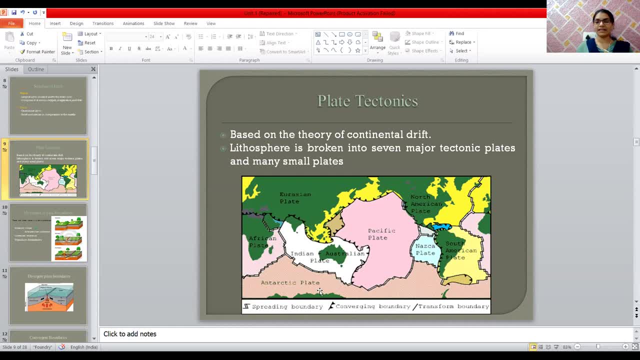 Separation Of Plates Are Occurs. The African Plate And Indian Plates Were Broken Up And Separately Was. Indian Plate Are Joined In The Plates. 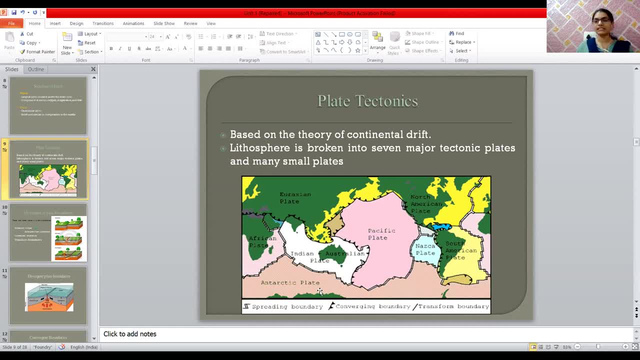 And The Plates Are Broken Into Seven Major Tectonic Plates. These Are The See The Diagram Was Naming, Like A Pangea And Ethos. 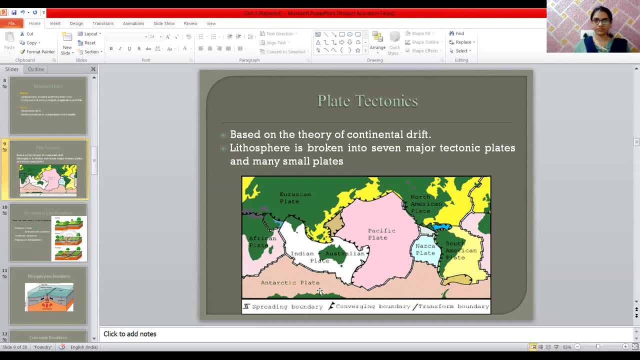 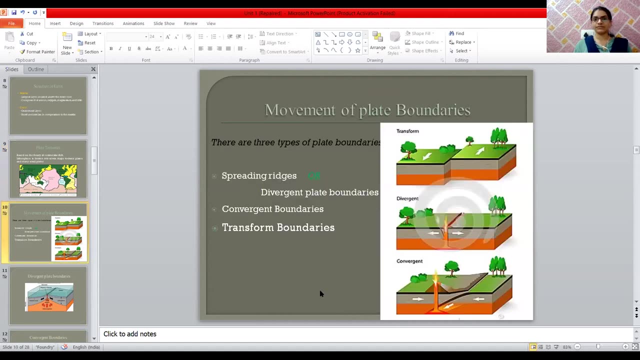 Period Broken About The Plate. Okay, Now About Discuss About Plate Boundaries. These Are The Three Types Of Boundaries: Borders Or Boundaries First. First. 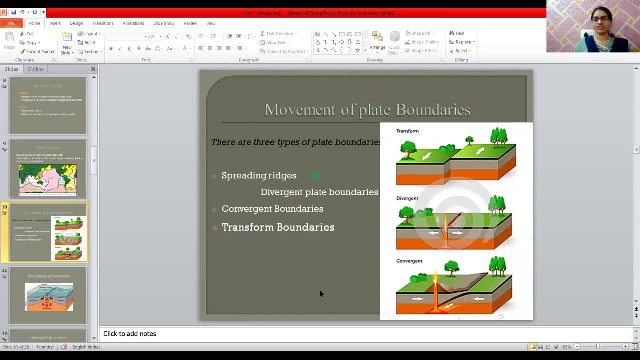 Boundary Borders Was Divergent Of Plate Boundaries. Next, Convergent Boundaries Are Moving Opposite Direction. Okay, The One: Tectonic Plates And Other. 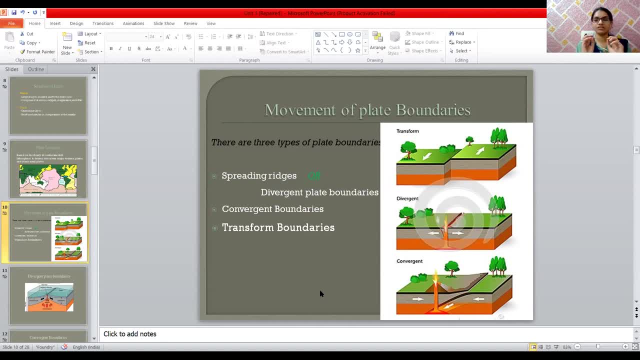 Tectonic Plates Moving About The Opposite Direction Is Called As Divergent Boundaries, Conversion Boundary, Boundary, The First Of Crust. Okay, These Are. 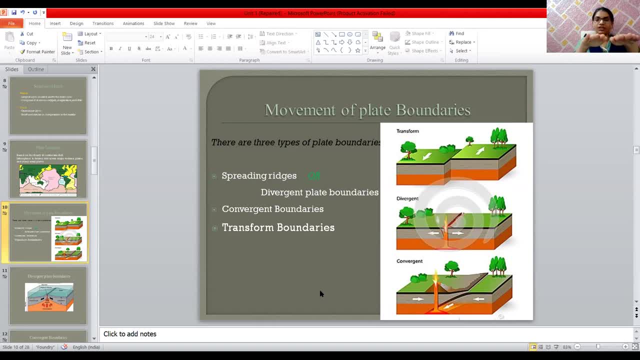 The Convergent Boundary, The First Boundary And Second Boundary. The First Boundary As Over The Second Boundary And The Next Boundary, Bottom Of Boundary. So 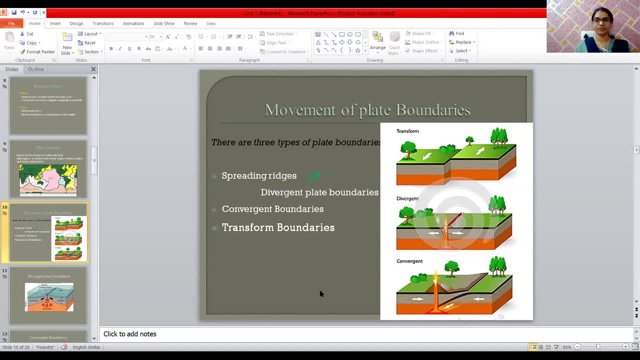 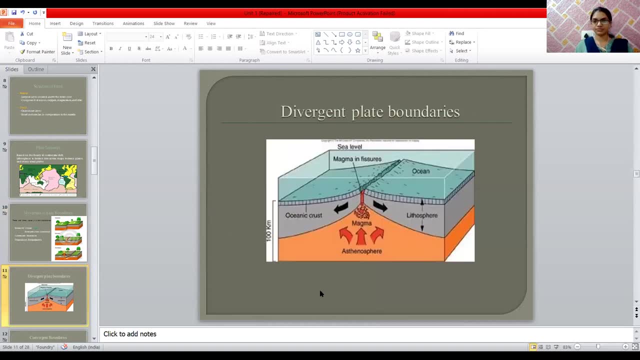 Now These Are Seen On The Diagram. Now Explain This Briefly. Like This Diagram, Magma Are Comes Into The Earth, Inner Most Part Of Earth. 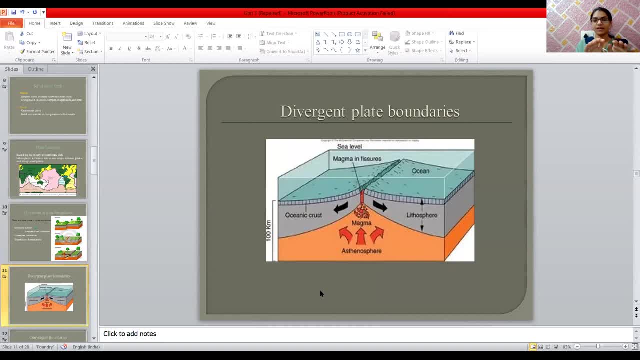 And Open In The Pansion Plate. Sorry, Tectonic Plates Are Broken Upon Two Parts, First Left Side Part And Then Second Is Right Side. 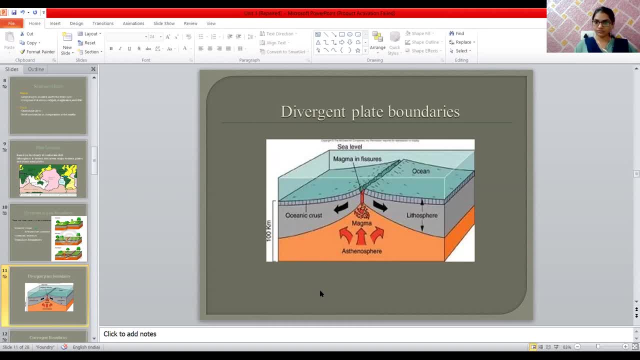 And Middle Parts Of Middle Part Are Broken And In This Two Plates Between The Two Plates Are Present Above Magma And These Plates Are 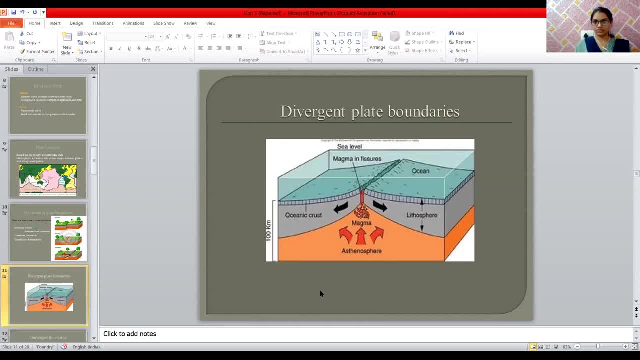 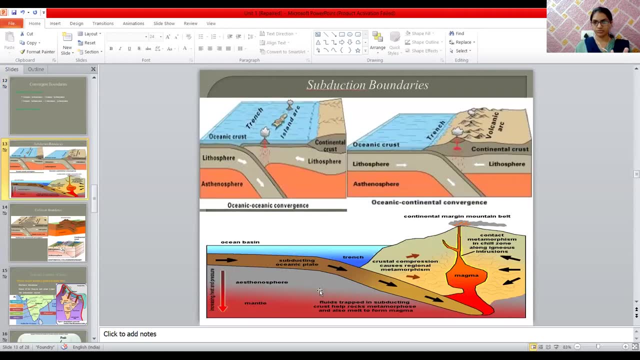 Moving Opposite Direction For Opposite, Opposite To Direct, Opposite To Directions. Okay, Next, Two Plates Are Broken, Broken Upon. Two Plates Are Broken And. 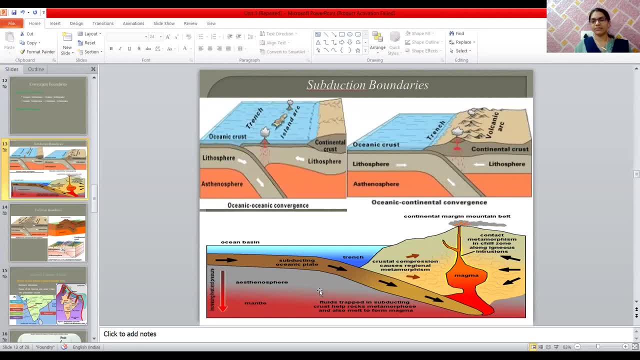 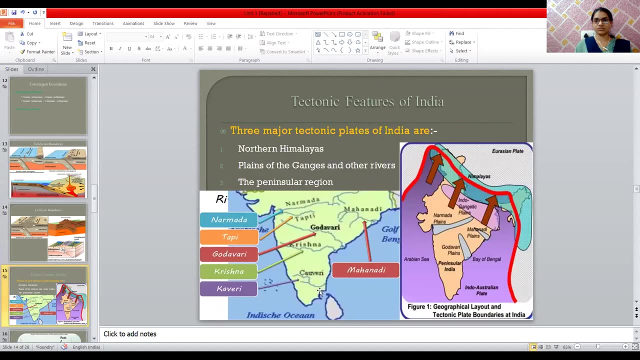 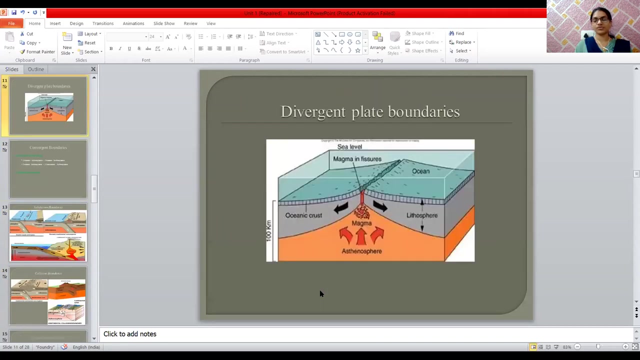 One Plate Is Downward To First Plate. Okay, See, In This Diagram There Seen About The First Plate. Next Transformation: Transform, Sorry, Transform, Boundary, These 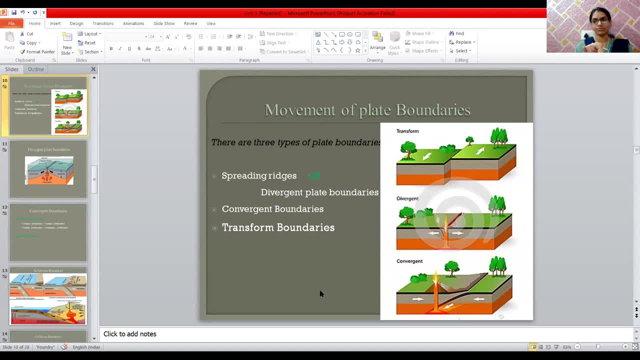 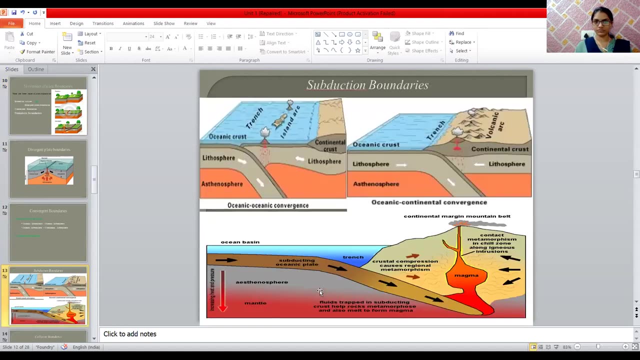 Are The Diagrams About Transform Boundary. There Are Two Plates Are Moving Opposite Direction And, As In This Opposite Direction, We Are About The 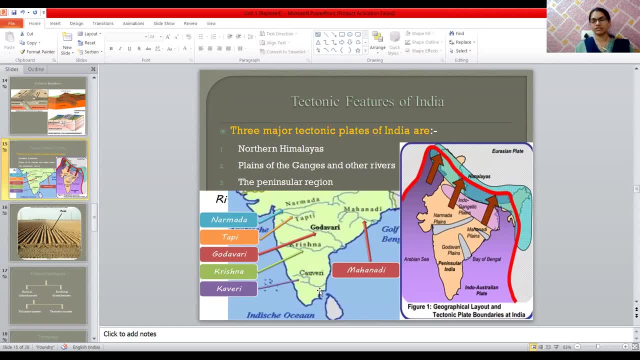 Tectonic Future Of India Same, For This Is Example Of Plate Tectonic. Sorry, Indian Plate Are Broken And Join To Asia The Him Himalaya. 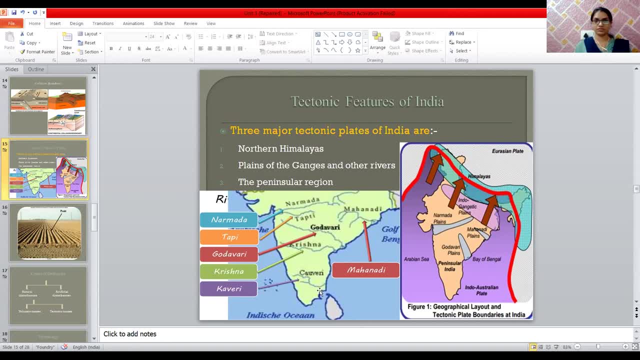 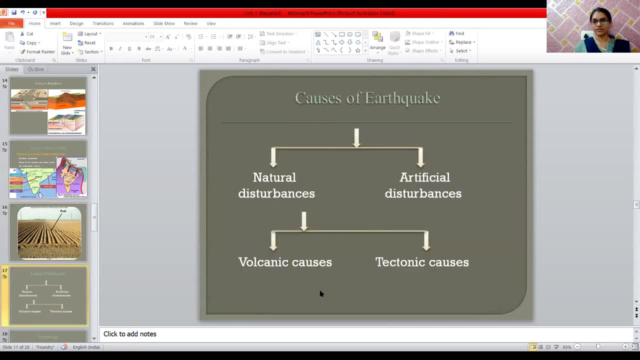 Range Was Developed. Okay, Next Course Of Earth, Wake. There Are Two Types Of Earthquake: Are Occur Natural And Artificial. Natural Earthquake Offers The 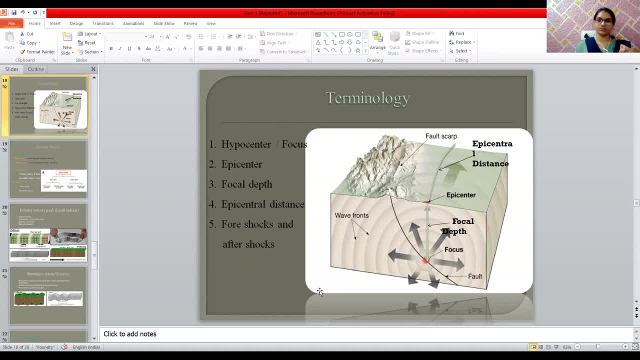 Volcano And Tectonic Plates. These Are The Most Common Definitions In This Earthquake. The First Of All. These Are The Five Definition Of Earthquake. 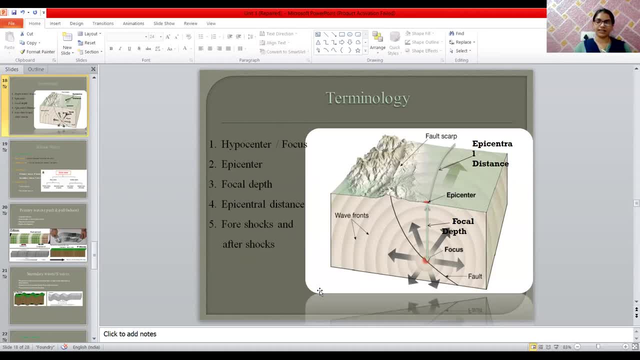 These Are First Focus, Second Epicenter And Third Focal Depth, Next Epicentric Distance. And For Earthquake Was Generated In The Ground, In The Ground. 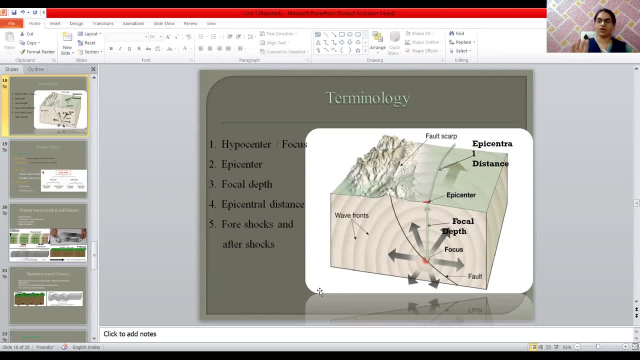 Earthquake Had Generated In The Ground. Then This Point, The Generation Of Earthquake, Then This Point Is Called As Focus, After The Top Surface Of 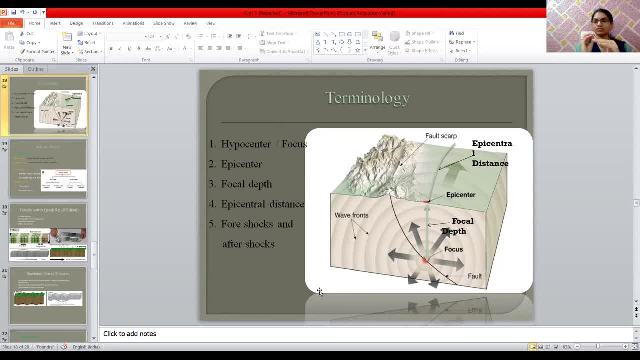 Earthquake, Sorry, Surface Of Earth, Then This Point Are Called As Epicentric. Then Now In This Diagram We Are Seen And The Distance Of This. 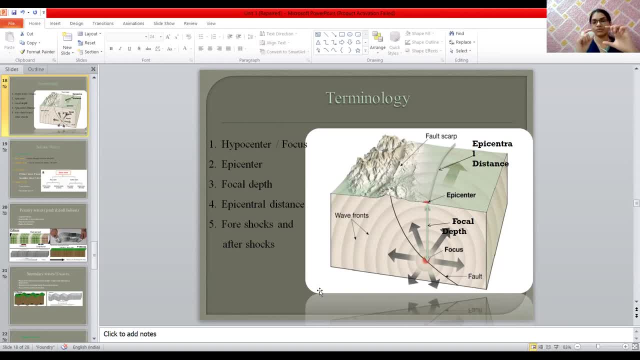 Point Is Called As Focal Depth. This Depth Are Also Called As Focal Depth. First. First Definition Was A Focus, Focus With Generation, Generation Of. 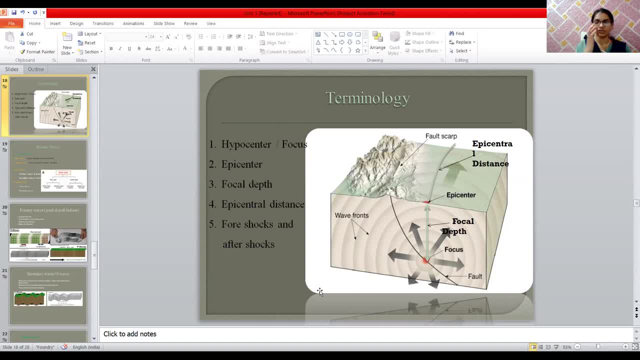 Earthquake, Okay, Generation Of In Under The Earth, Sorry, Under The Ground, Focus And Topmost In Crust, The Distance Of Focus And Epicenter Was: 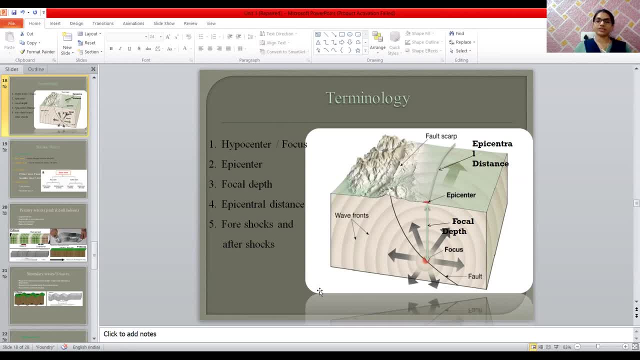 Focal Depth And The Epicenter Was Straight Of Focus Distance Was In This Diagram, Epicentric Distance Was Epicenter To Focal Okay And The 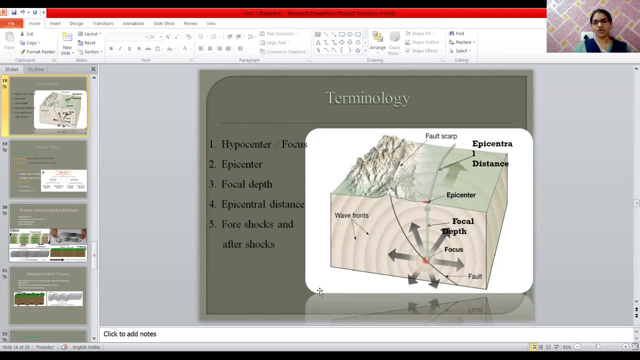 Next Force Shock And After Shock. Force Shock Means Of Force Earthquake: Sudden Occurs In Earthquake. So We Are Discussing About This Definition. 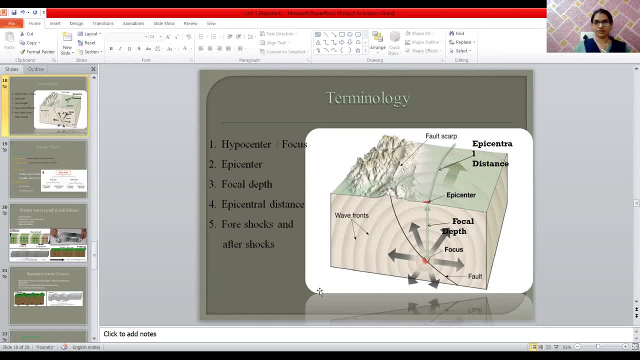 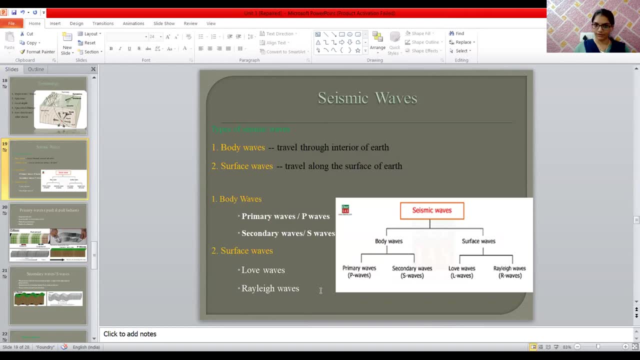 This Is About The Next. We Are Discuss About The Seismic Waves. There Are Two Types Of Waves: First, Body Wave And Surface Waves. The 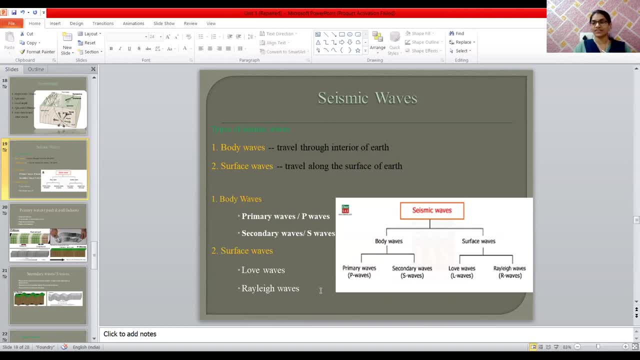 Body Waves Are Also Divided Into Body Waves. So First Of All, We Are Discussing About The Body Wave. Body Wave Travels In Inner. 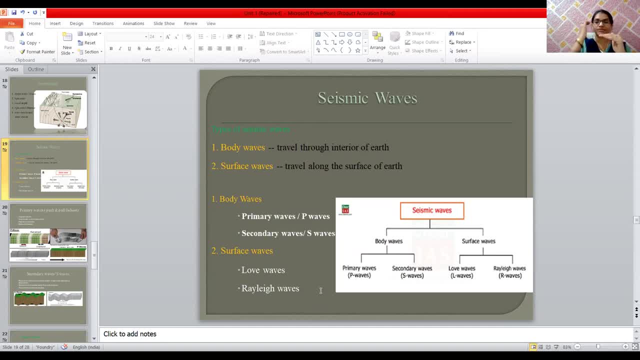 Most Part Of Earth. Okay, The Difference Between Body Wave And Surface Wave There Are. Body Wave Are Also Two Divided Into Two Types: Primary: 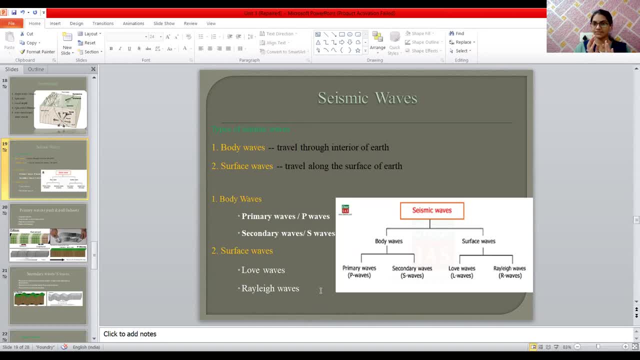 Wave And Secondary Waves Are Also Called As Wave, Then Surface Wave. Surface Wave Are Also Called As L Wave And Relay Wave Are Also Called. 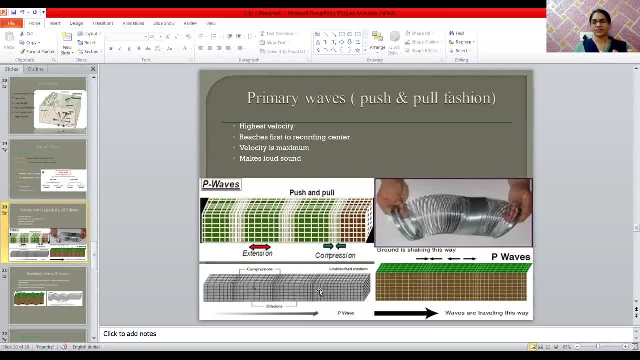 As R Wave. Okay, First Of All, We Are Discussing The Primary Wave, Or The Primary Wave, Or Then It Is Recording, For It Is. 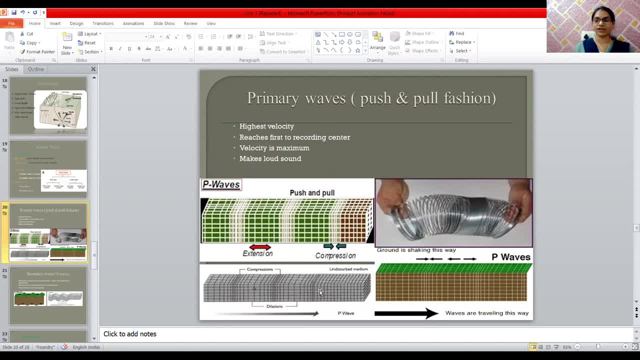 Recorded, Firstly Because The For Systemogram Are Recorder Meter For Earthquake Measurement. For This Is The First Wave Was Recorded Into The Sound, Sound Wave. 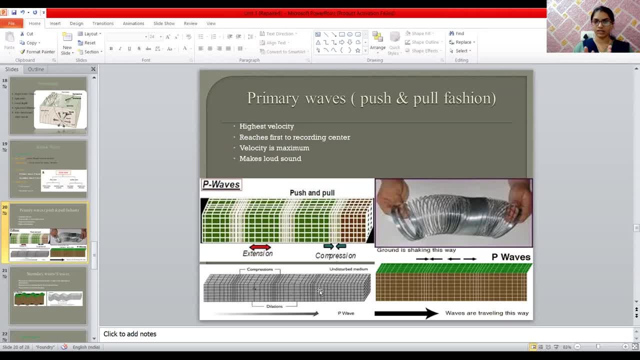 Like Structure Is Compression And Tension. Members Expression Sorry: Expansion And Compress. Compression Like A Structure. The Waves Are Passing. These Are In This Diagram. 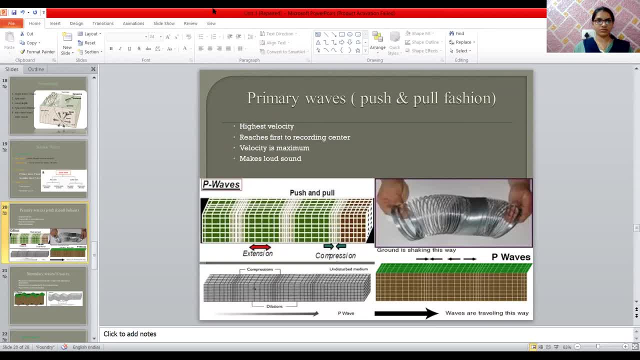 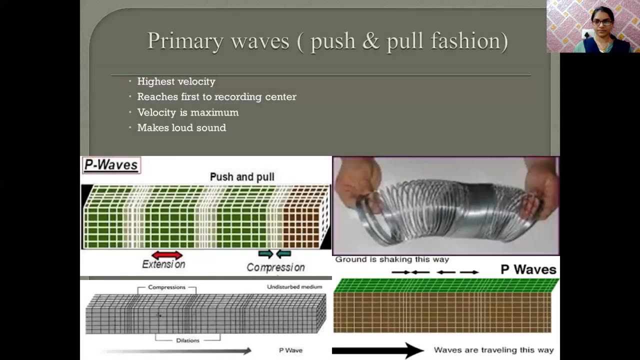 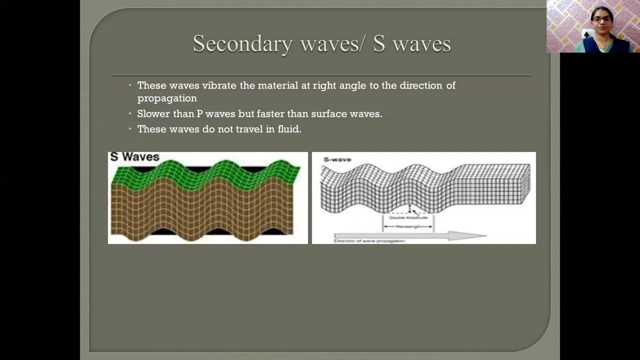 Push, And One Once, One, One Next, As If What You Mean By Secondary Wave The Those Wave Vibrates, Vibrates And Mental For Right Angle. 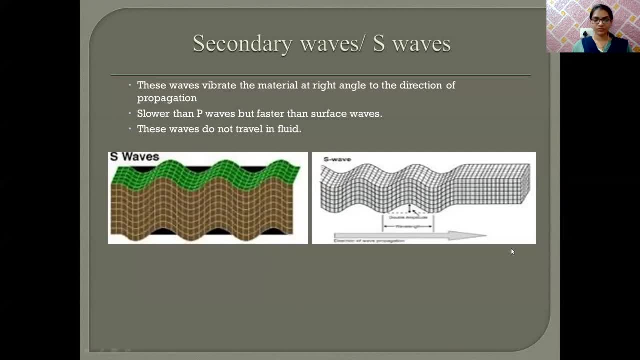 To The Direction Of Propagation. This Is Rope Like Structure. Roping Like Structure And As Wave Are Slow, Faster, But Faster Than As A Surface. 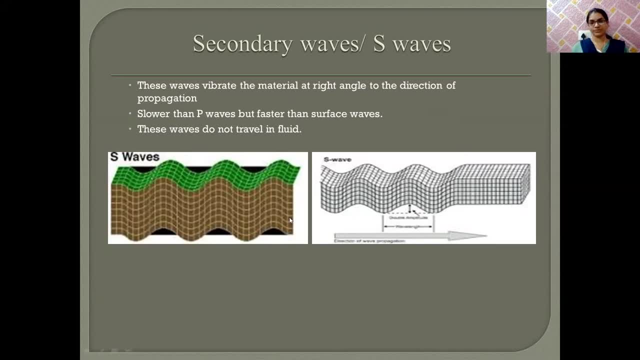 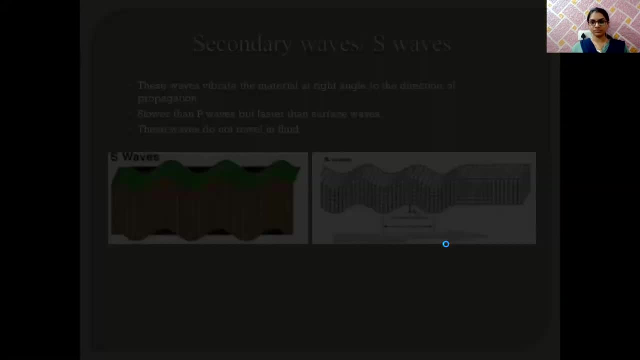 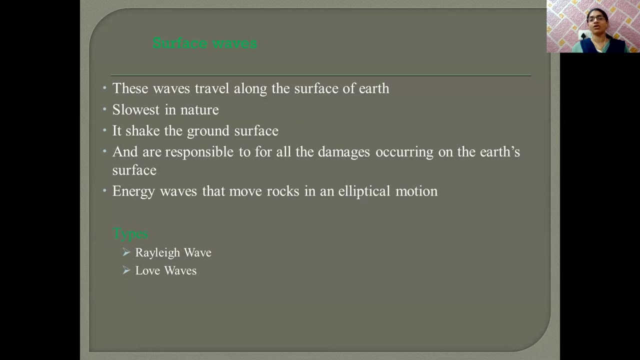 Wave And It Is Not Traveling About Fluid. Now The Diagram Was Seen. Now Surface Wave- Surface Wave: Does The Wave Travel In Nature? It? 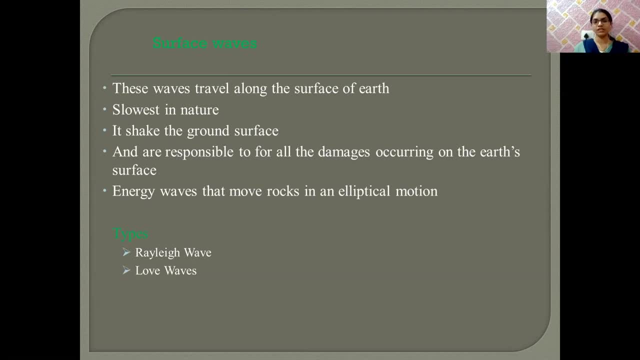 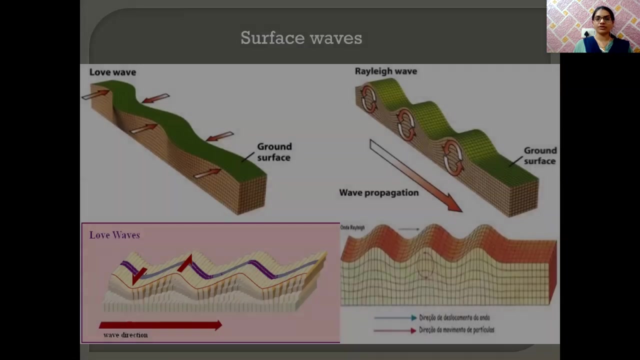 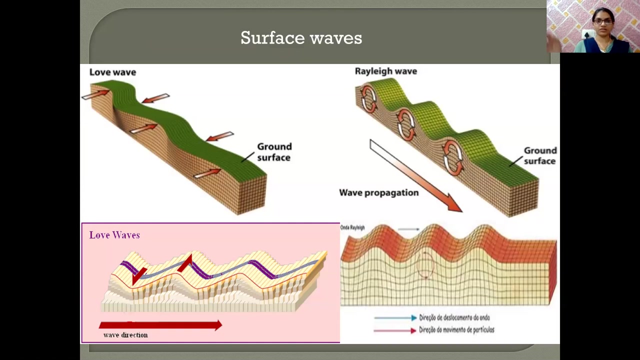 Shock Of Ground Surface. The, It Is Shock About The Ground Surface And It Is Energy Wave Moves To Shock In Epicentric Motion. There Are 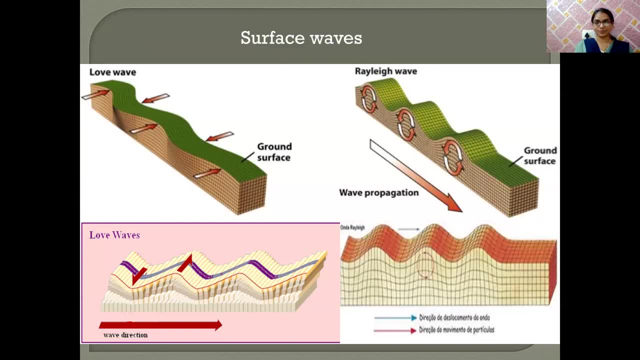 Two. These Are The Two Different Diagrams About Section The As Wave Are Similar To Narrow Curve. That Curve Like Direction In Horizontal Move Movement. 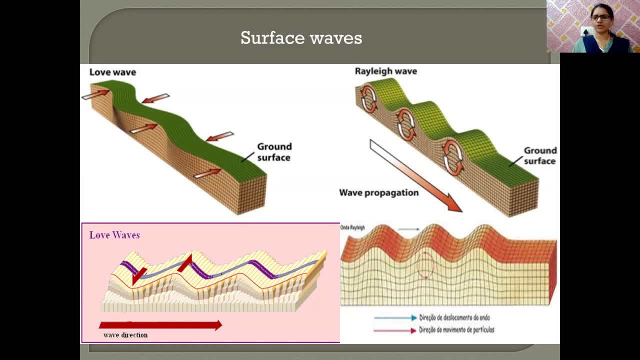 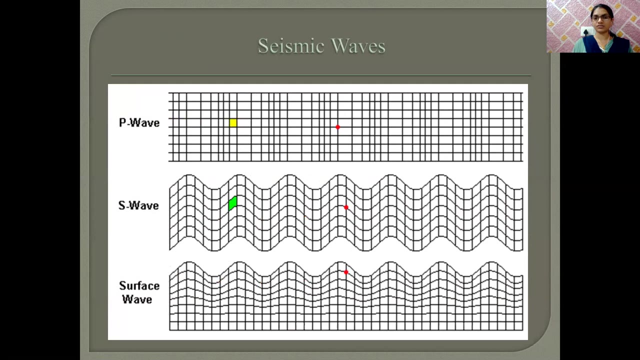 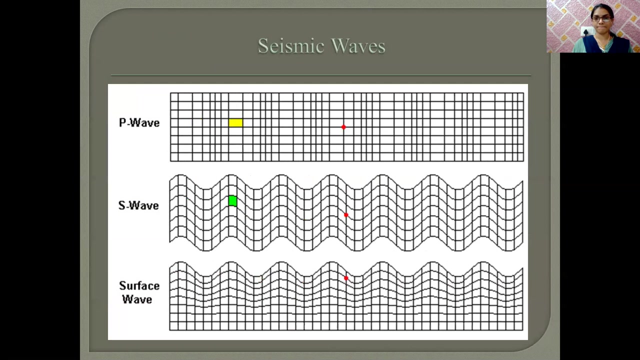 Of Ground And Top, Or A Rounded Like Structure, Rounded Motion Like Structure. Okay, Relative, These Are The Waves We Are Discussing About. Further These: 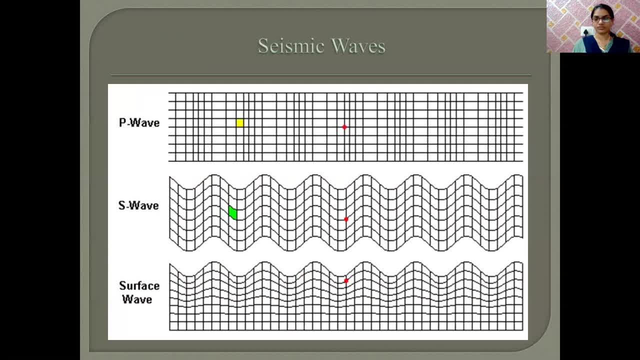 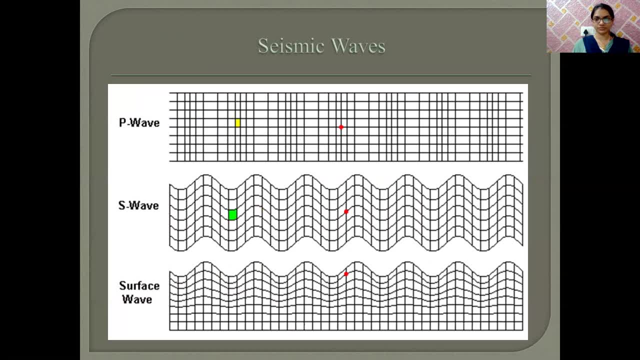 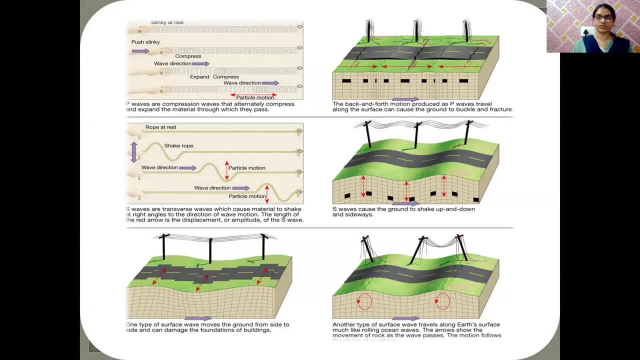 Are The Propagation Of Waves Okay, Same. This Is Diagram About Waves. Next Topic Was Sismo- Sorry, Sismic Zoning Of India. There Was A 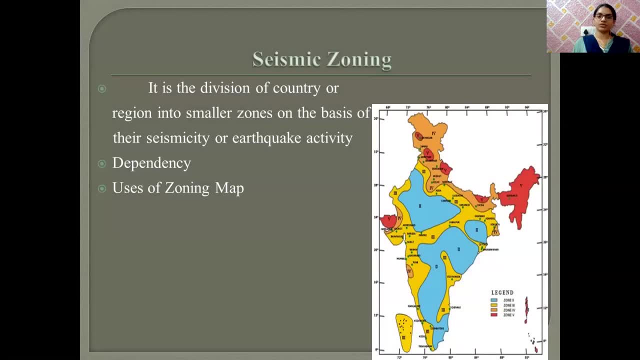 Five Type Of Zone, According To, Is The Zone Of Swimming Or The When It Has Back Scored One, Eight, Nine, Three, Two Thousand Two. 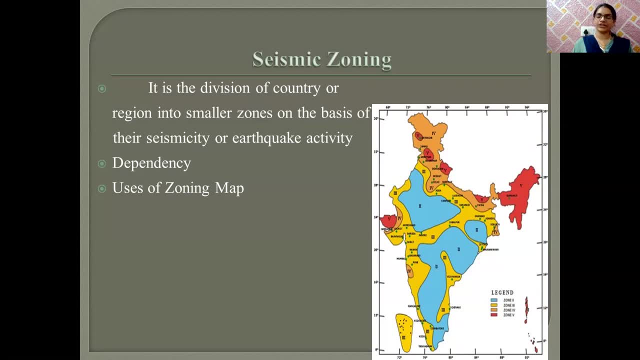 Five, Four, But Now A Day's, The Zone Between. Nowadays This Was About Four, four and five zone. These are the mapping of map about India and these are the region about zoning. under the map It is divided into the country or region of similar zone. 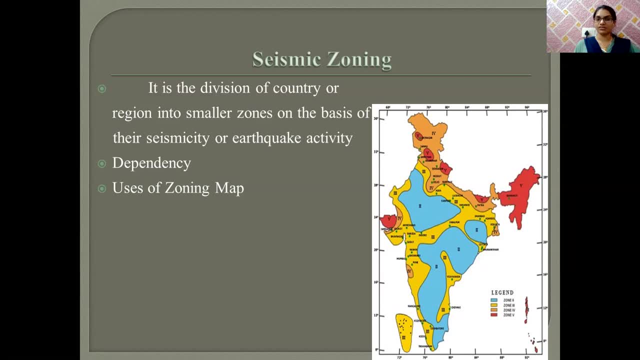 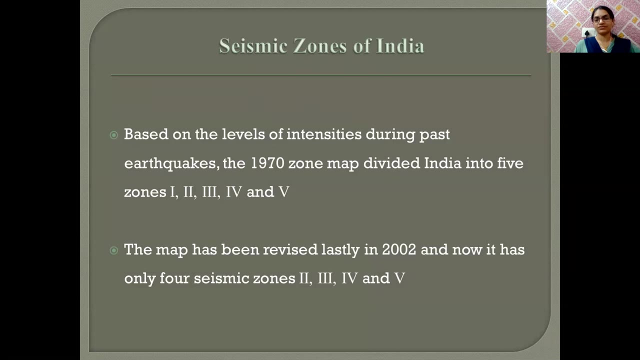 on the basic of the seismic seismicity or earthquake quality. Next basic level of intensity was during the past earthquake in 1970. zone map divided, divided India into the five zone: First, First, 2nd, 3rd, 4th and 5th. Then mapping about last earthquake in 2002 in Bhuj, they revised. 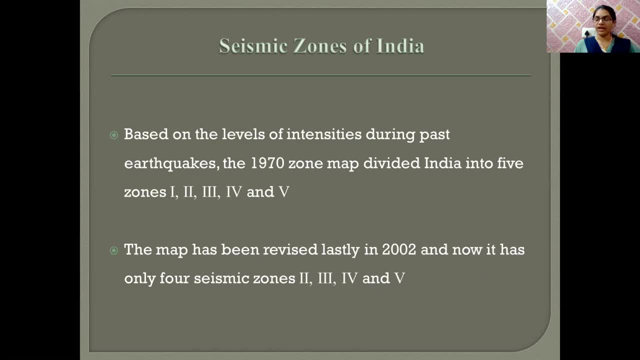 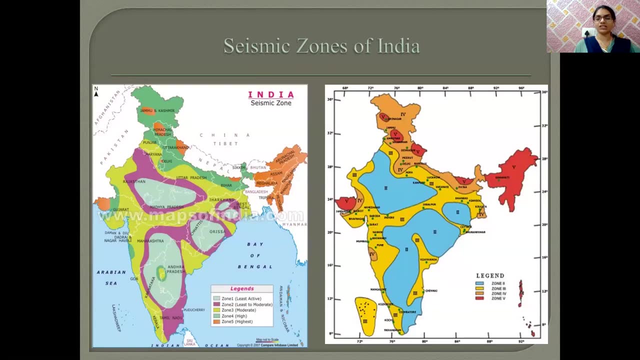 the zone like 2,, 3,, 4 and 5 only See. these are the 2 diagrams. about 1st diagram. we are seeing the zone 1st, 2nd, 3rd and 5th and these are the 2nd diagram. these are the revised. 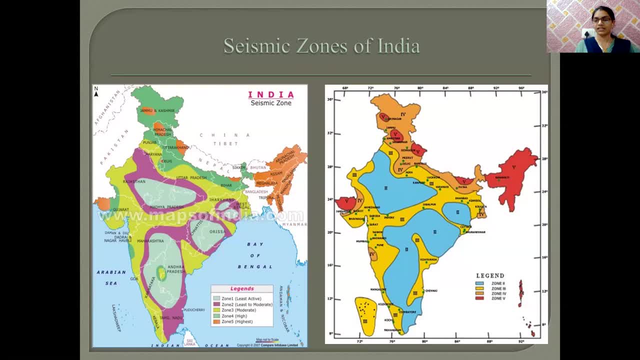 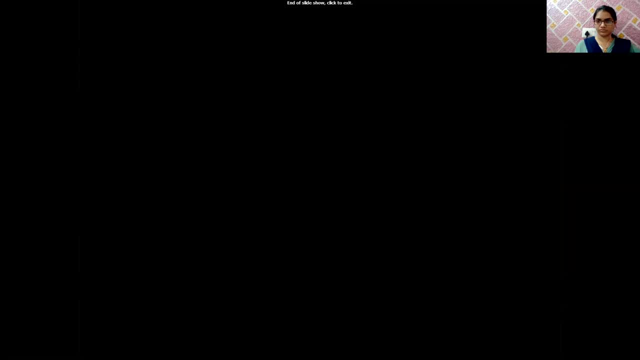 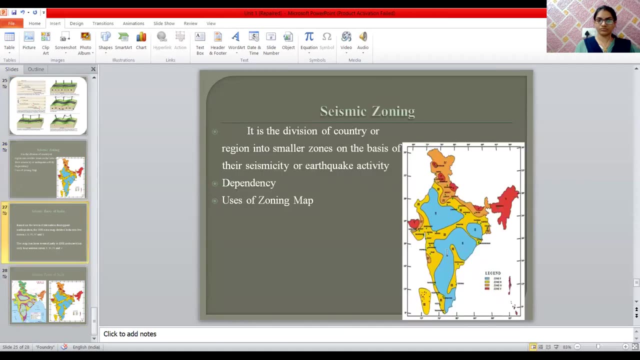 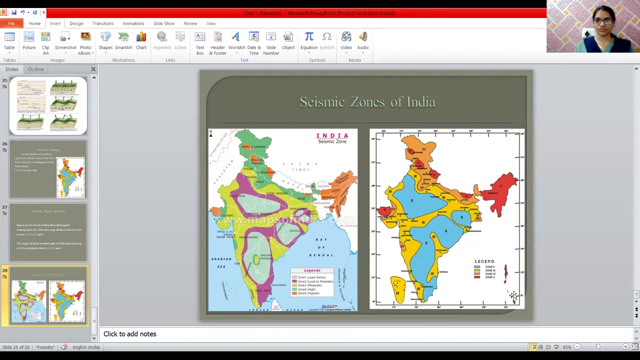 mapping: See these are the 2nd, 3rd, 4th and 5th. See these are the 2nd, 3rd, 4th and 5th.